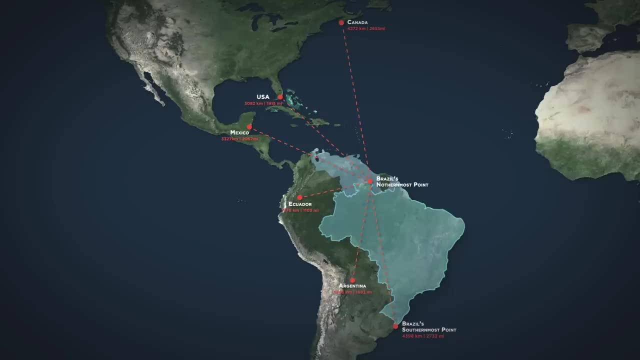 Brazil's northernmost point is, in fact, closer to every single other country in the Americas than it is to Brazil's southernmost point, a fact that defies most appeals to common sense. But even more shocking than that is this: What geographic location do you believe is the northernmost point of Brazil? 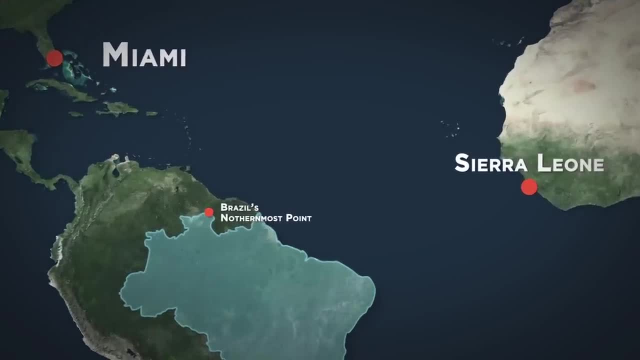 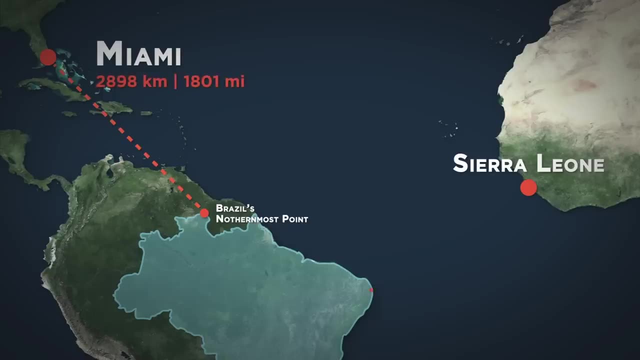 And what geography do you believe is closer to Brazil, Miami or Africa? So, starting again at the same northernmost point of Brazil, the straight-shot distance over to Miami is 2,898 kilometres as the crow flies, but Brazil's easternmost point over here is only 2,883 kilometres away from Sierra Leone across the mid-Atlantic. 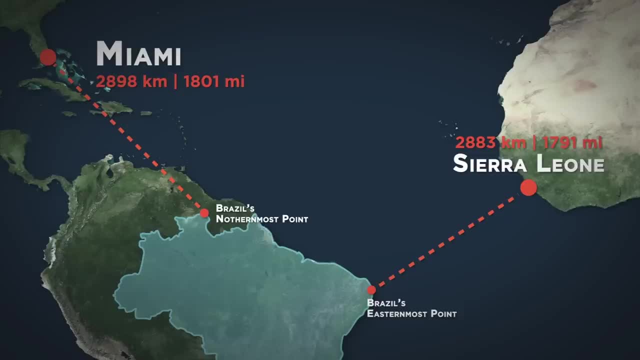 which means that Brazil is located a very narrow 15 kilometres closer to Africa than it is to Miami. Brazil's northernmost point is locations at twoOST. Basically, bring your какой flèches retail 들어� high whenever you're going to the US. You'll notice that the Northern and Atlantic regions have been completely, completely dismantled, See. they're all usually exeKay种ated, but that means that nobody gets the general give way into the ballpark of the mid-Atlantic region, See, Brazil is certainly the northernmost point across the habitable South Africa and the midas and South Africa region. than it is to Miami, meaning that you can factually say that Miami is further away from Brazil than Africa. The biggest reason for why this may come as a surprise to you is because most of us in the Northern Hemisphere have a weird misunderstanding of where exactly South America is located geographically. 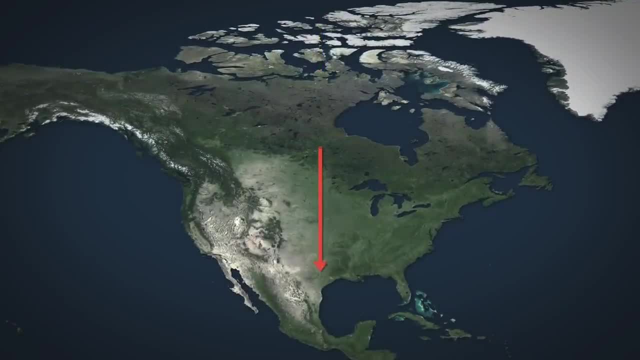 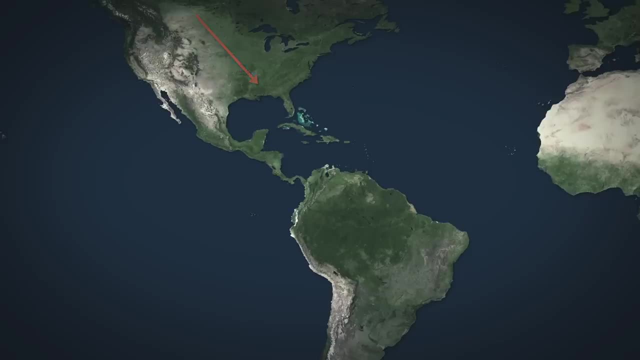 We all know that South America is, of course, south of North America, but it's easy to forget or simply not know that South America isn't directly south of North America. If you're in the United States and look south and you draw a straight line down from your gaze. 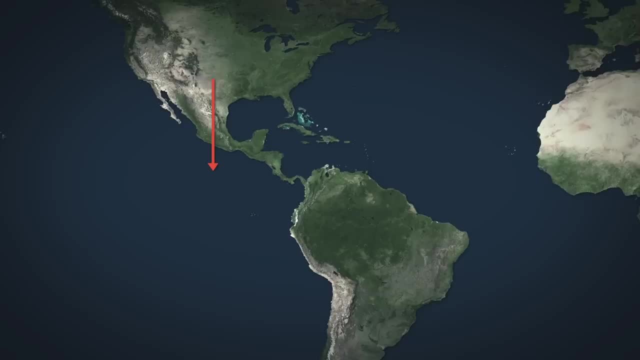 it's unlikely that that line will ever actually hit South America. This is because if you start in Jacksonville, Florida, and draw a line straight down across the globe, you'll discover that the entire South American continent lies just to the east of this line. 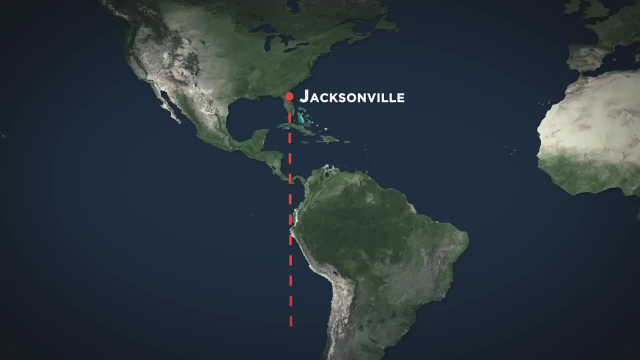 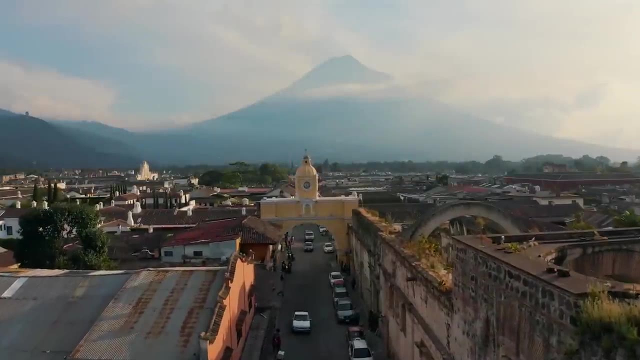 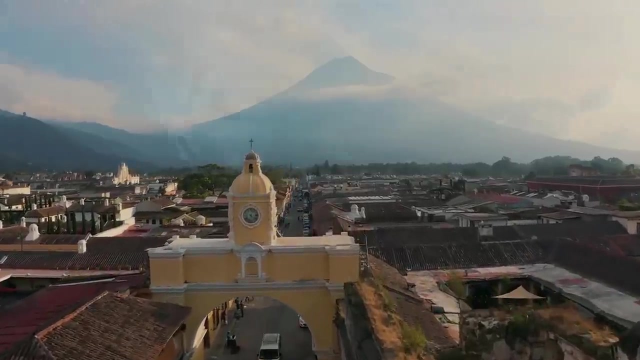 South America is so far east that the entire continent is significantly east of Detroit and therefore most of the United States. South America is much further east than North America, further east than most of us believe it to be in our heads, and because of that there's some other interesting geographic implications. 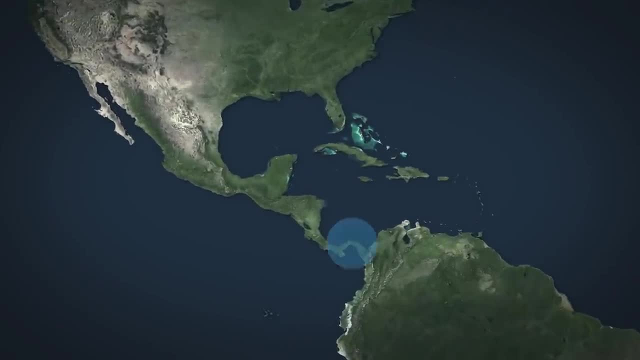 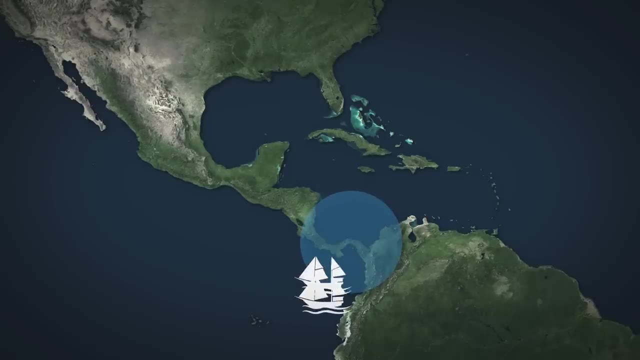 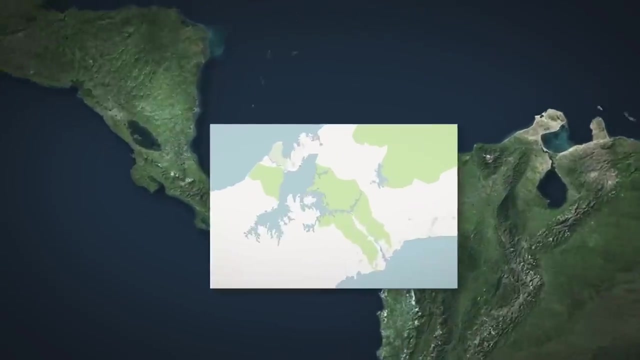 Despite not being strictly located in South America, the Panama Canal is close enough to warrant some mention here. The canal enables ships to travel between the Western Pacific Ocean and the Eastern Atlantic Ocean quickly without having to sail all the way around South America. But if you zoom in closer to the canal itself, 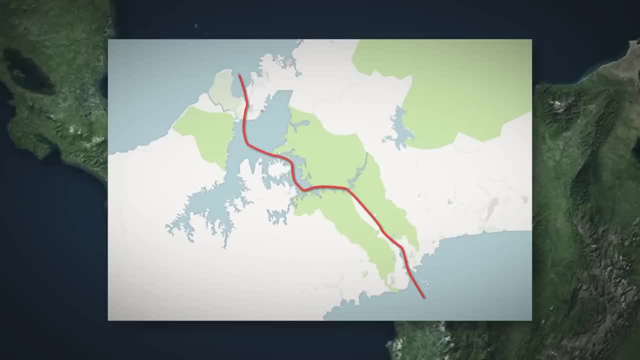 you discover that ships travel through it in a rather unexpected direction. If you're starting in the Eastern Atlantic Ocean and you're going across the canal to the Western Pacific Ocean, you actually begin in the north and generally travel southeast to reach the Pacific. 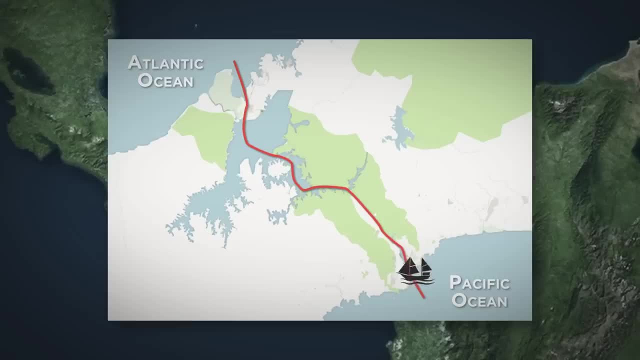 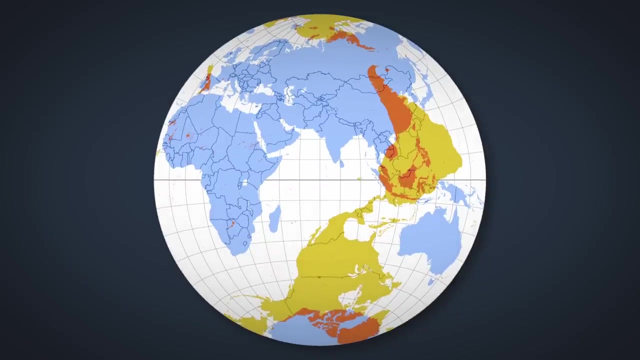 To further complicate your confusion, the Atlantic side of the canal is actually further to the west than the Pacific side is, which means that to travel from the Atlantic to the Pacific you actually end up traveling east. South America is so far southeast that it's actually on the exact opposite side of the world from the Pacific. 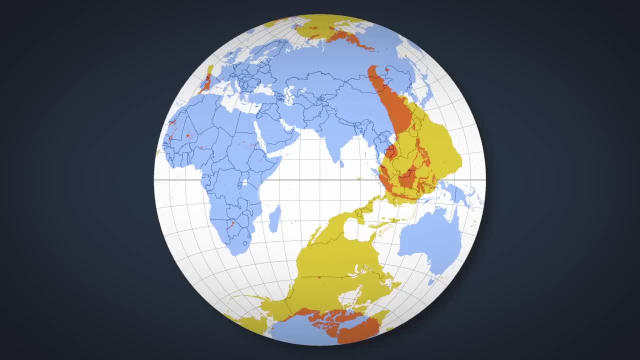 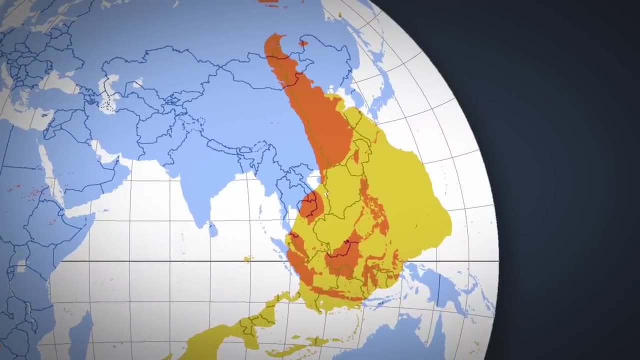 South America is so far southeast that it's actually on the exact opposite side of the world from the Pacific Asia. If you began anywhere in South America and dug a hole straight down to the other side, here is a map showing you where you'd end up popping out at If you began in Argentina or Chile. 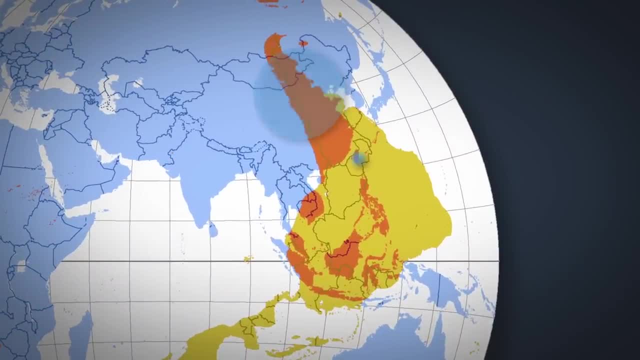 you'd end up somewhere in Siberia, Mongolia or China, Paraguay would get you into Taiwan, Peru would cause you to wind up in Vietnam, Cambodia or Malaysia. Brazil would get you into the Philippines or Indonesia, while Colombia, Venezuela, Guyana, Suriname and French Guyana would all end up putting you. 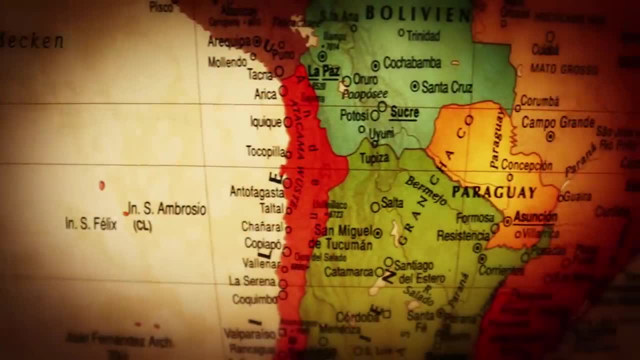 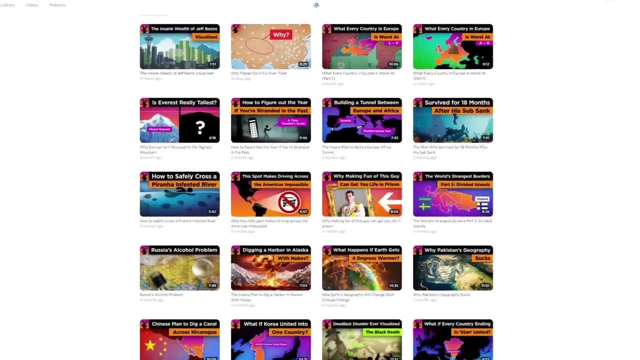 across the various islands of Indonesia. So yeah, South America's geography is probably a little weirder than you might have thought it was. Now, if you've made it this far in a watching, then you probably love real-life lore, and I'm sure that you've probably already heard all about CuriosityStream, the documentary streaming service that has 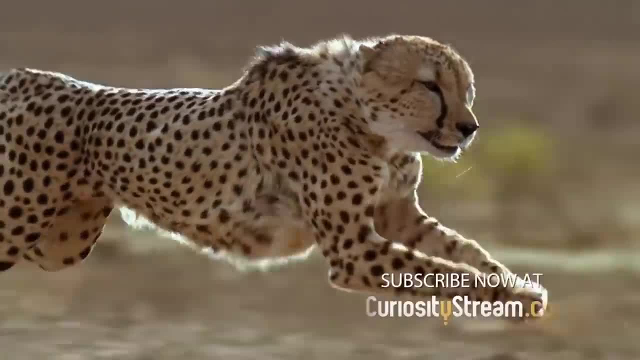 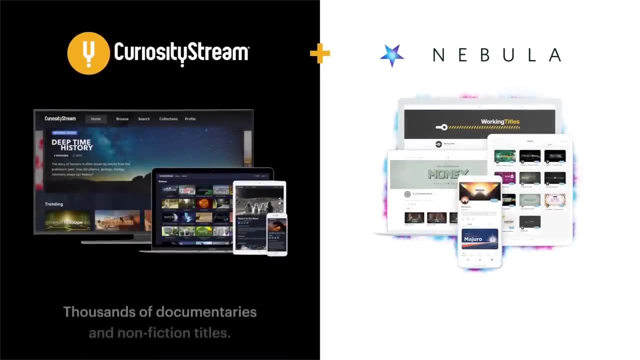 thousands of videos on geography, history, engineering and tons of other things, But thanks to CuriosityStream, when you sign up for them, you'll also get access to Nebula, a streaming service made by educational creators like me, where we can publish our original. 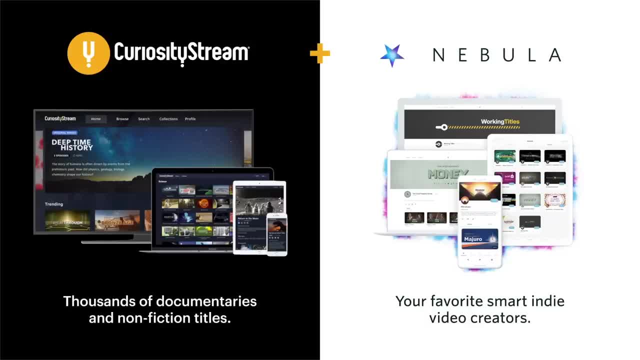 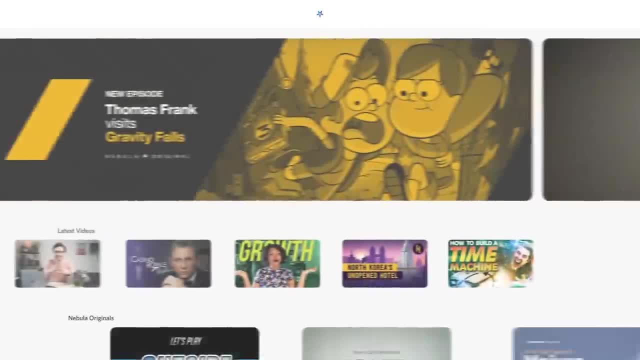 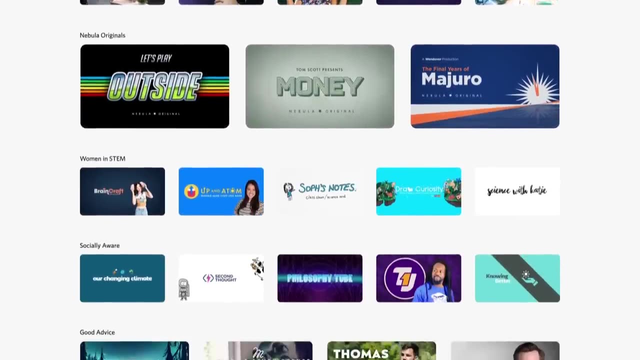 thoughtful content without fear of getting demonetized or buried by YouTube's dreaded algorithm. By signing up for CuriosityStream and Nebula, you are directly empowering me and dozens of other educational creators you probably know- to make cool, exclusive content that we might not ever get the chance to make otherwise. 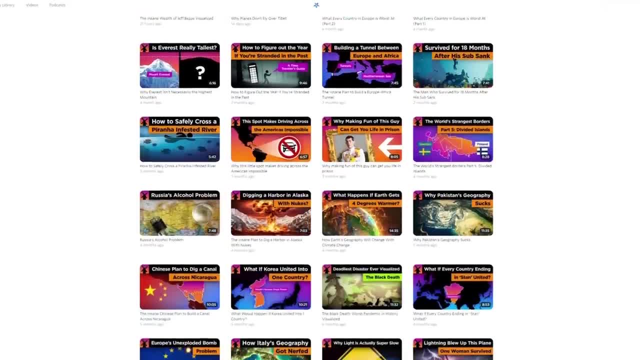 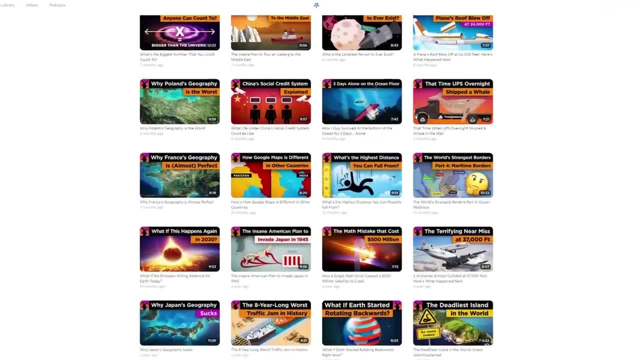 Content like all of my own real-life lore videos that go up at least 24 hours early before they ever do on YouTube, and all without any ads or sponsorships. And exclusive content like money, a game show hosted by Tom Scott and featuring a bunch of my creator friends in a series of psychological